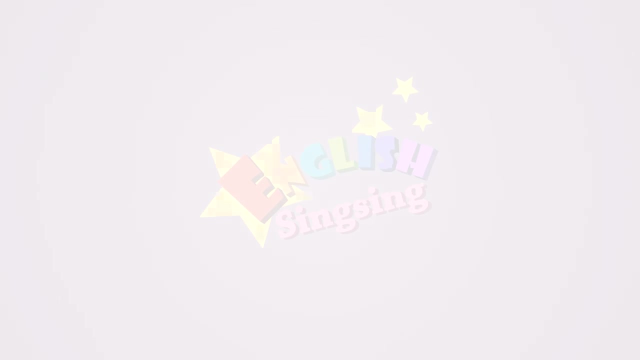 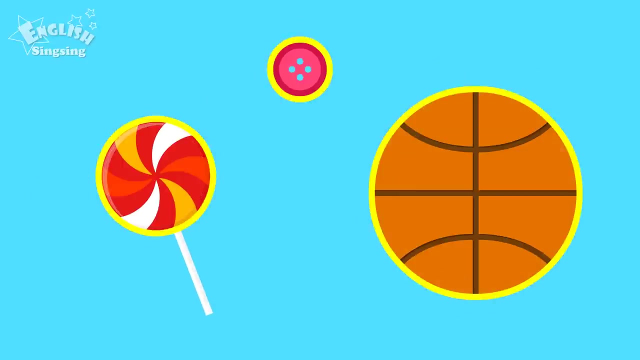 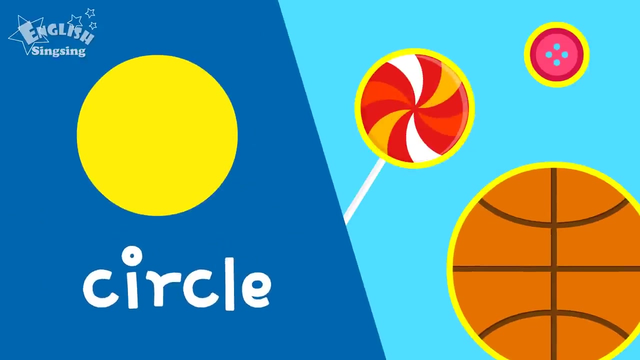 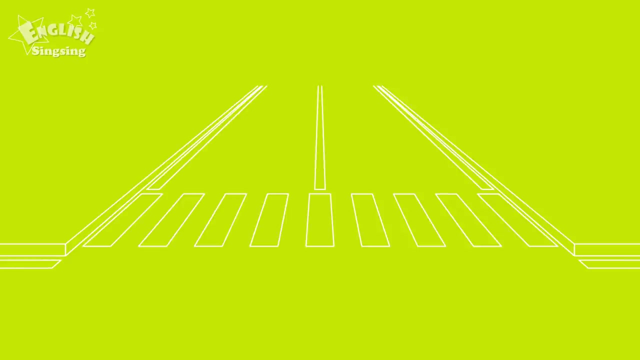 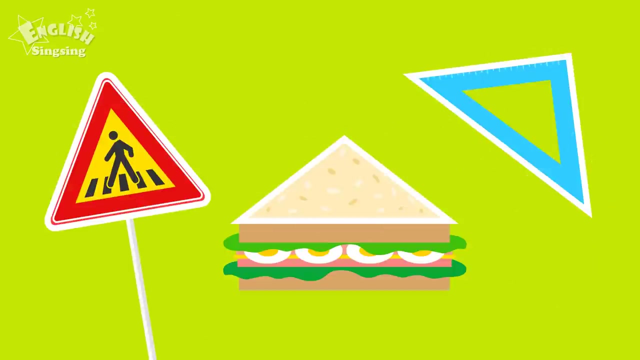 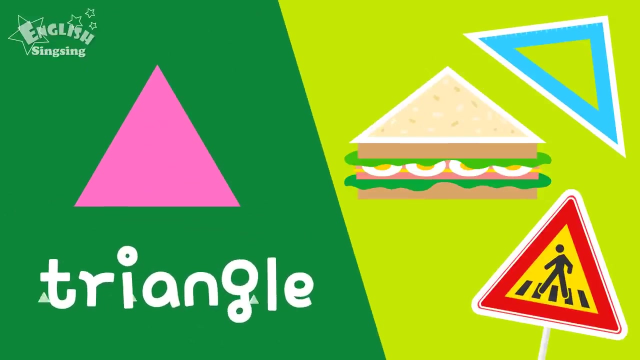 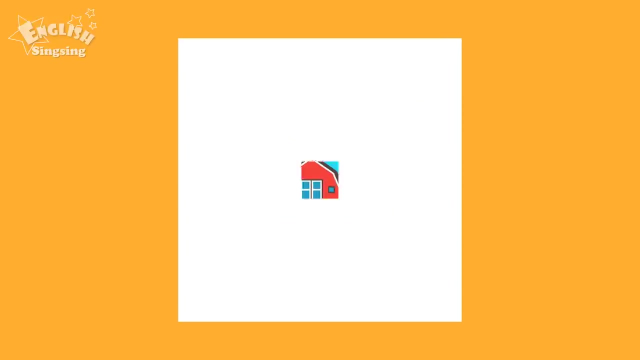 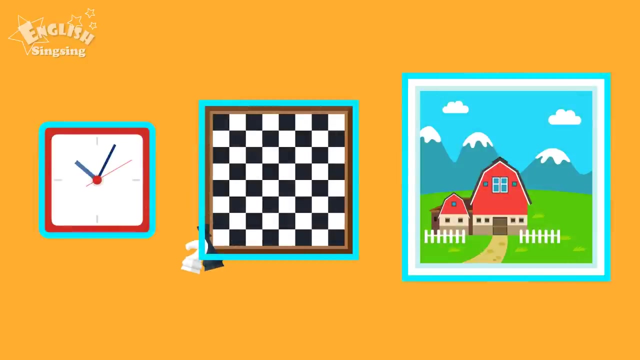 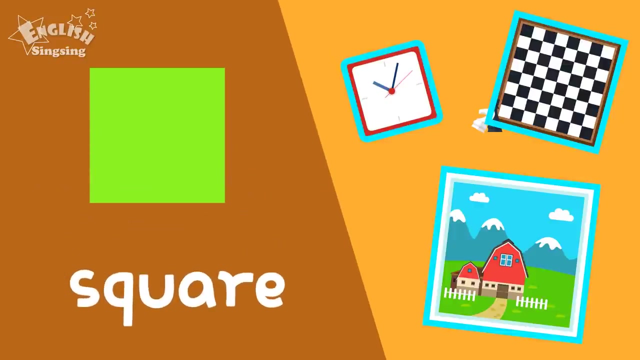 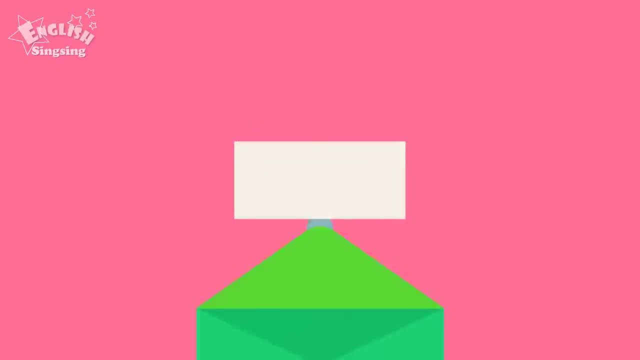 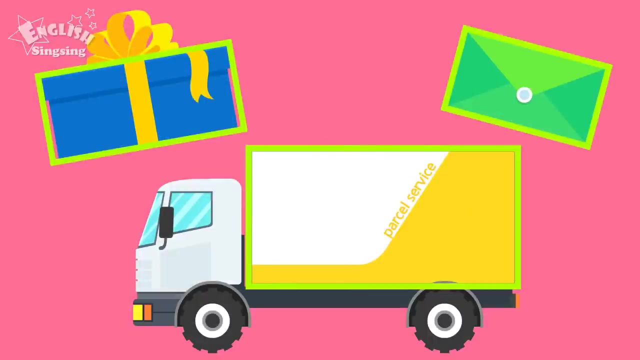 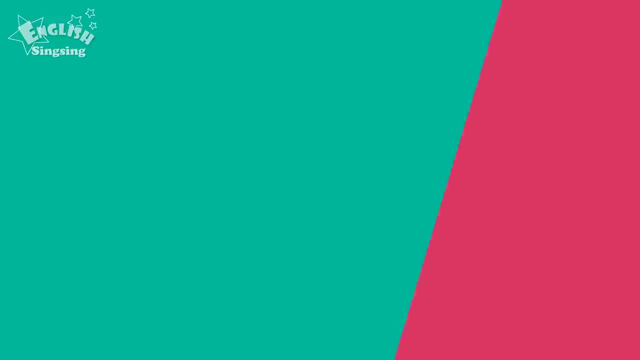 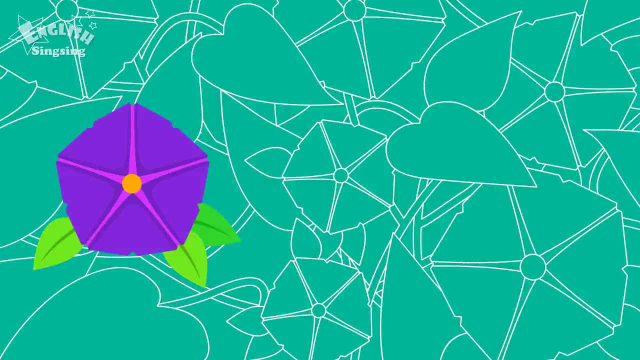 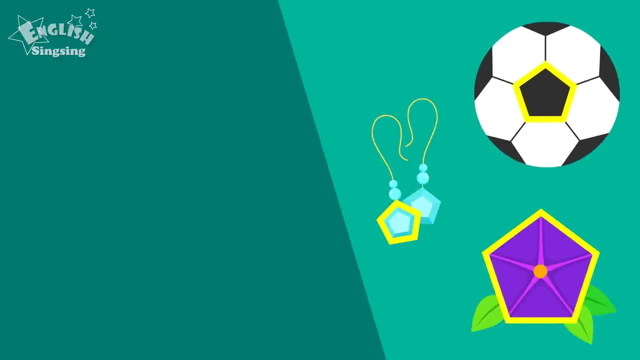 English, Singsing shape. These shapes are circles, circle, circle. These shapes are triangles. These shapes are triangles, triangle, triangle. These shapes are squares, squares, square, square. These shapes are rectangles: rectangle, rectangle, rectangle, rectangle. These shapes are pentagons: pentagon, pentagon. 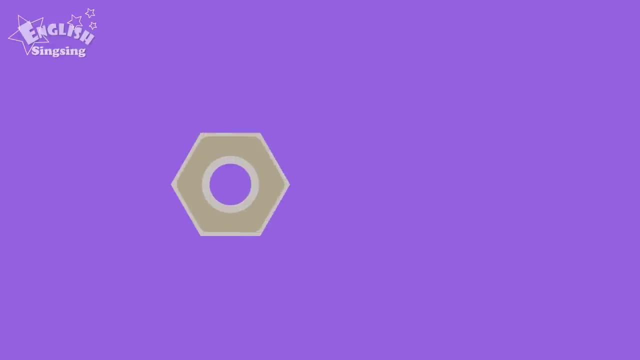 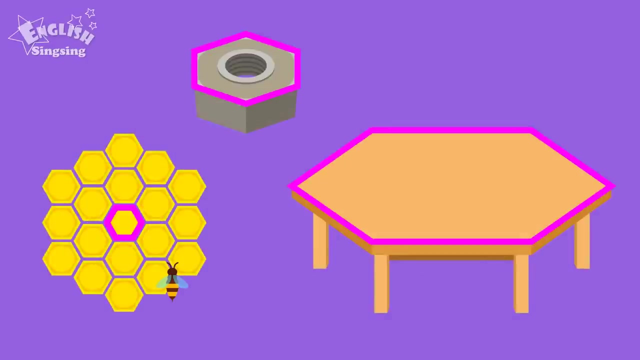 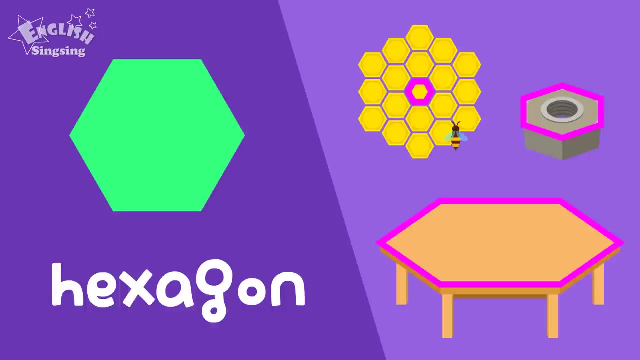 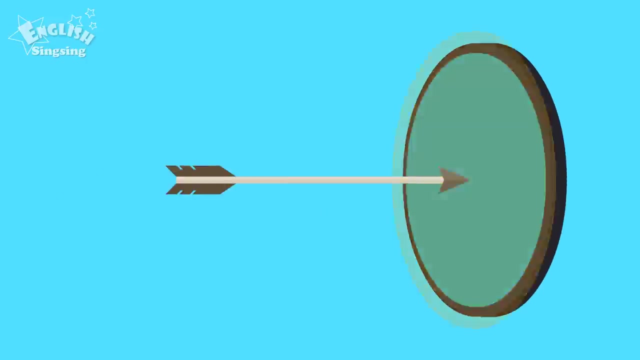 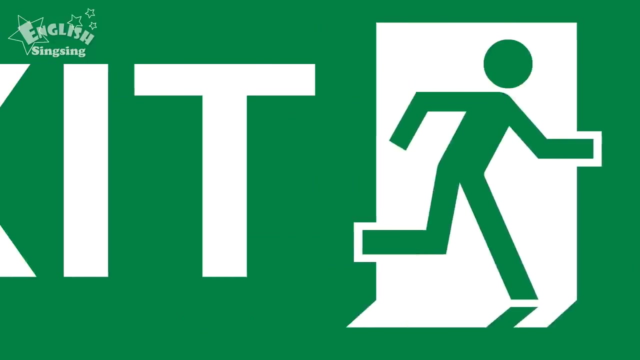 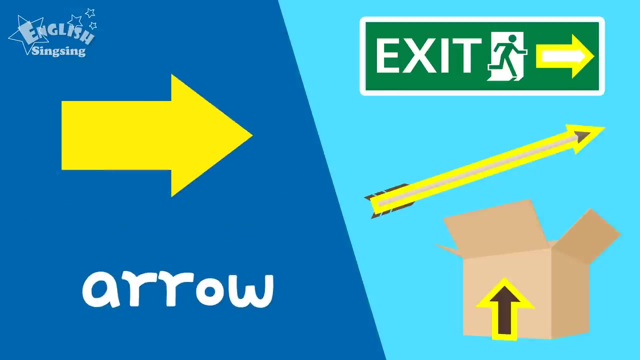 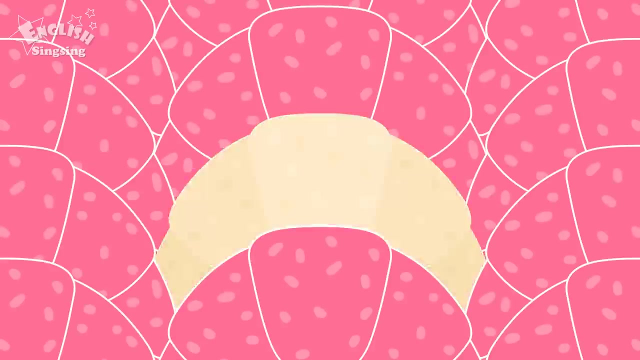 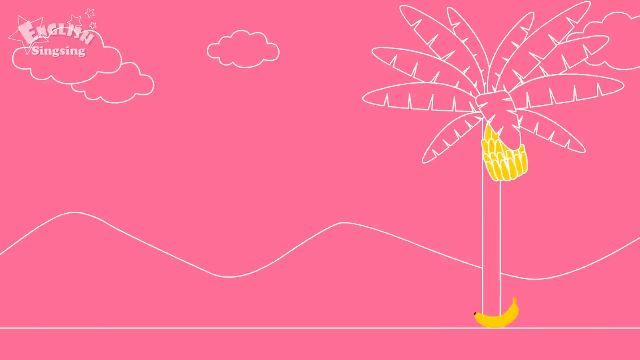 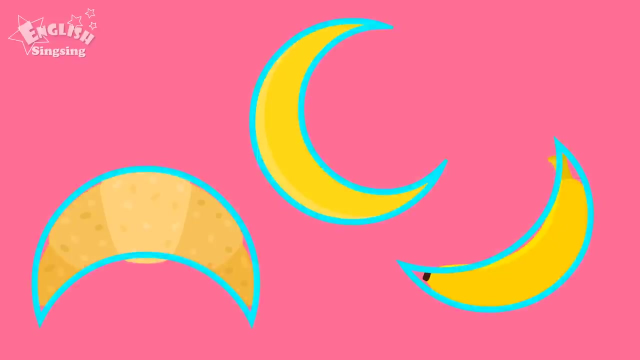 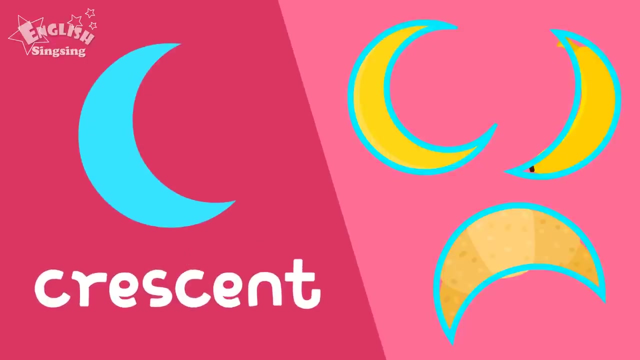 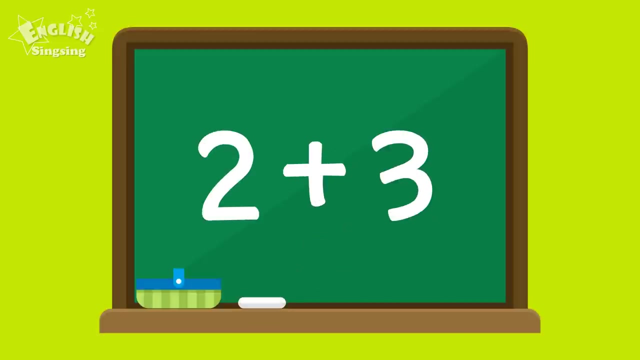 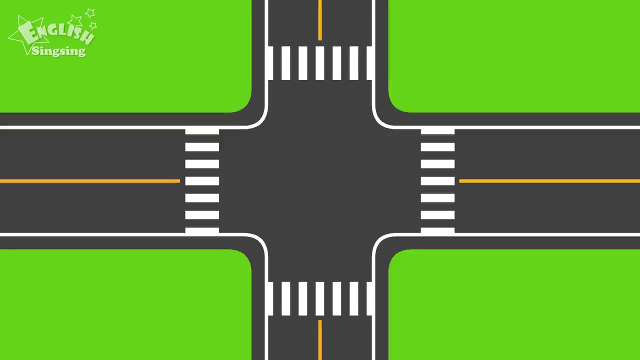 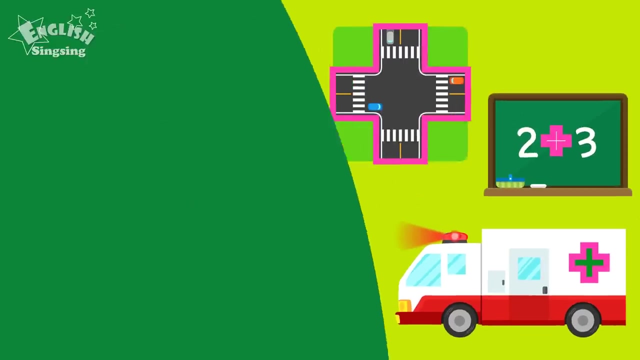 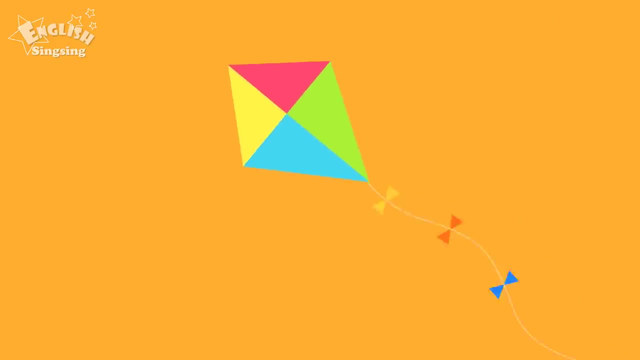 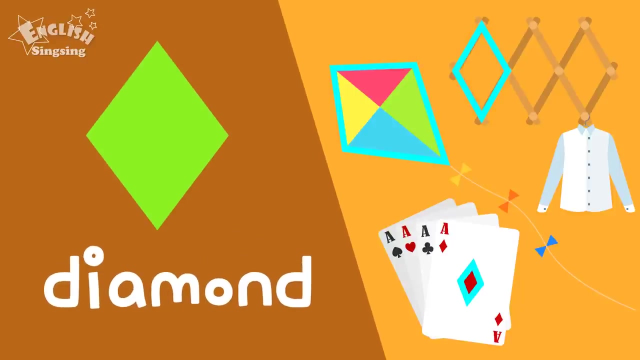 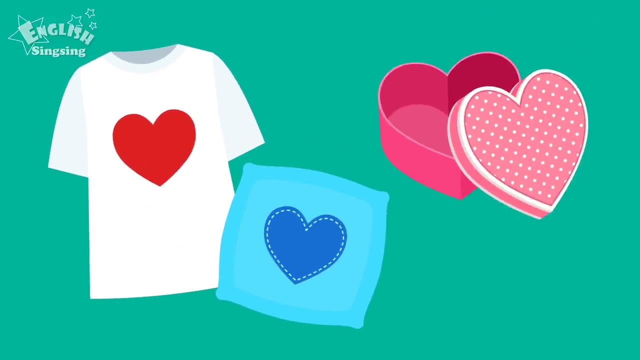 pentagon, pentagon, pentagon, pentagon. These shapes are hexagons, hexagon. These shapes are arrows, arrow. These shapes are crescents, crescent, crescent, crescent. These shapes are crosses, cross, cross. These shapes are diamonds: diamond, diamond. These shapes are hearts.